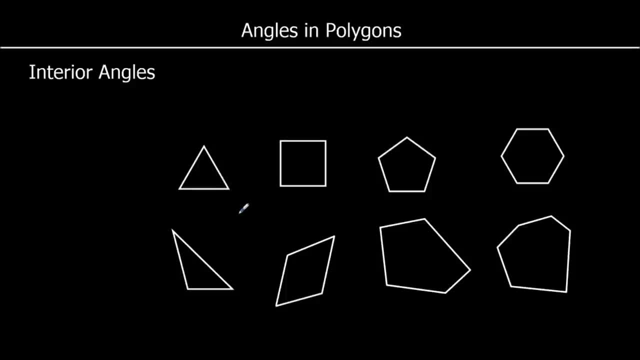 look different to the ones on the bottom and that is because they are regular polygons. That means that every side is equal. So in this regular triangle, an equilateral triangle, we've got three equal sides and three equal angles In the regular quadrilateral. 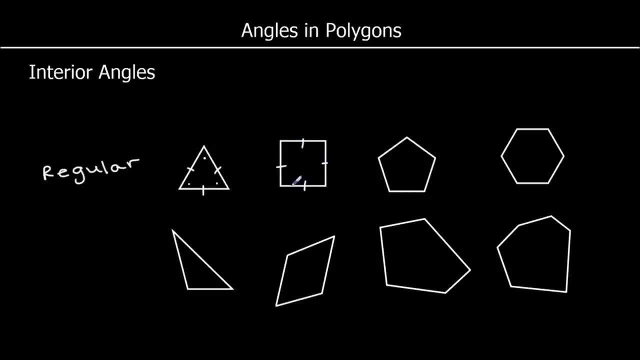 which we call a square, we've got four equal sides and four equal angles And again in the regular pentagon, five equal sides and five equal angles. So we've got regular shapes and irregular shapes. So irregular shapes don't have equal sides and 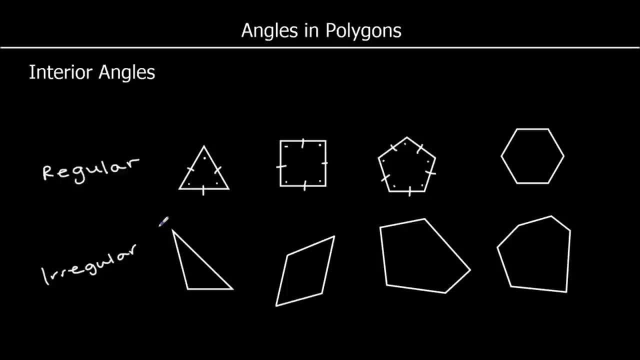 angles And in regular shapes all the sides and all the angles are equal. So we've got a three-sided, a four-sided, a five-sided and a six-sided shape, And let's look at their angle sums. Let's look at what. 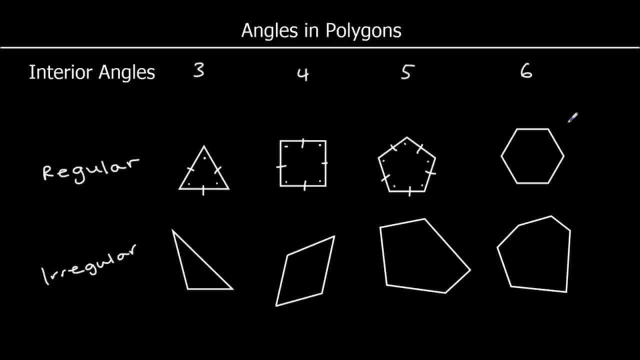 the angles in them add up to. So the angles in the triangle add up to 180 degrees. The angles in a quadrilateral add up to 180 degrees. The angles in a hexagon add up to 360 degrees. The angles in a pentagon add up to 540 degrees. 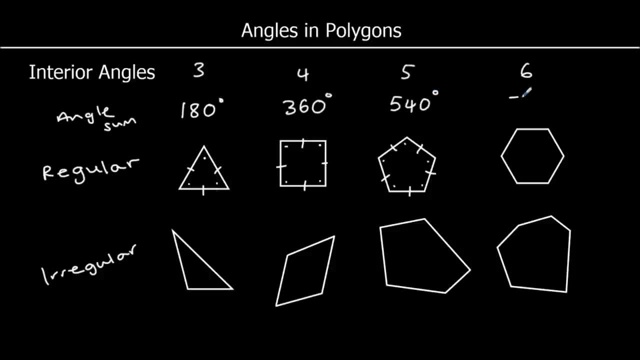 And the angles in a hexagon add up to 720 degrees. So you might notice there's a pattern here. It goes up by 180 degrees every time. So we can say: a quadrilateral can go up by 180 degrees. A hexagon can be split into two triangles, two lots of 180.. 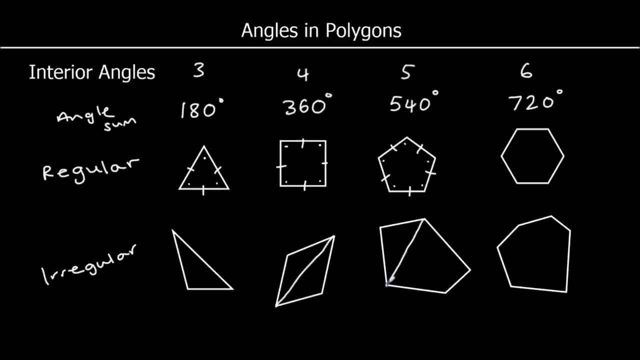 A pentagon can be split into three triangles, three lots of 180. And a hexagon can be split into four triangles, which is four lots of 180.. So to find the angle sum of a polygon, we can take the number of sides. 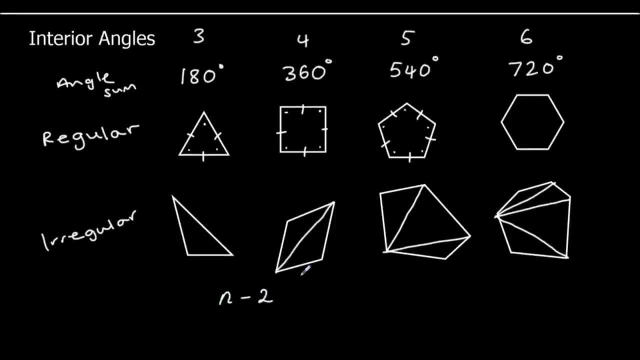 Which we'll call n, take away two And then multiply by 180.. So for a triangle, three take away two is one, so one lot of 180.. For a quadrilateral, two lots of 180, four take away two. 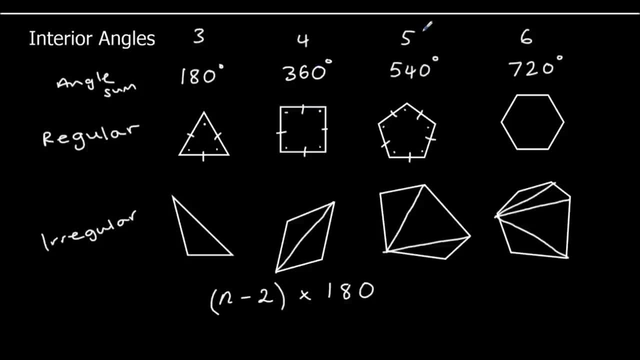 For a pentagon, three lots of 180, which is five, take away two. And for a hexagon, 6 take away 2 is 4, so it's 4 lots of 180.. So this is the angle sum of a polygon. 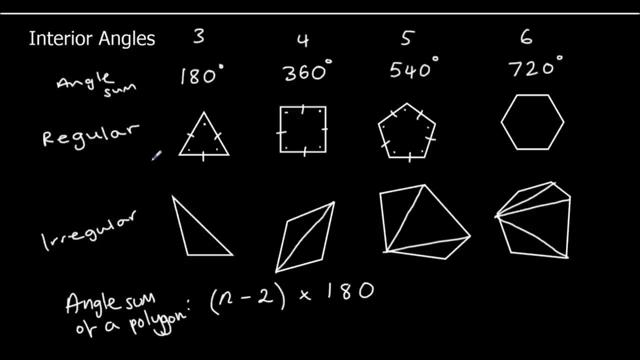 If we've got a regular polygon, we know that every angle in it must be equal. So for a regular triangle, an equilateral triangle, if we do 180 divided by 3, we get 60. So we can say that every angle in a regular triangle is 60 degrees. 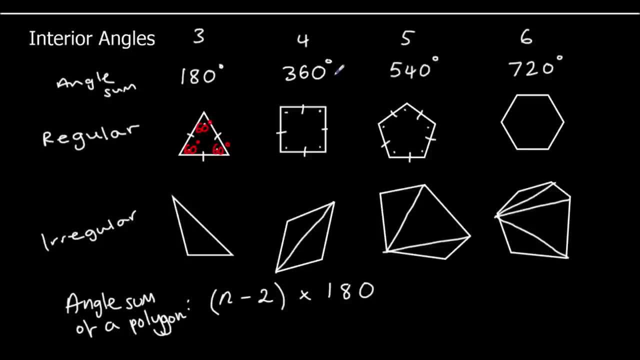 If we did 360 divided by 4, we would get 90.. So we can say that every angle in a regular quadrilateral or a square is 90 degrees. If we did 540 divided by 5, we get 108.. 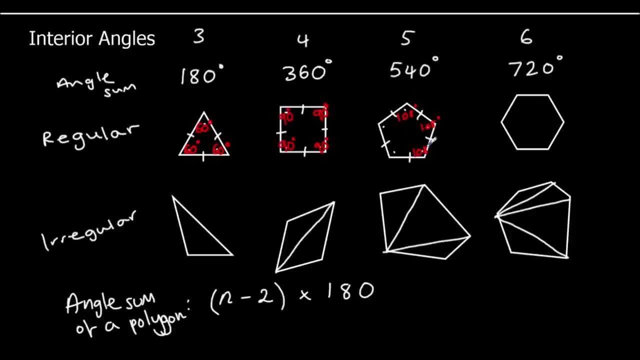 So we can say: every angle in a regular pentagon is 108 degrees. And if we did 720 divided by 6,, what would we get? So 720 over 6. It's the same as 360 over 3,, which is 120. 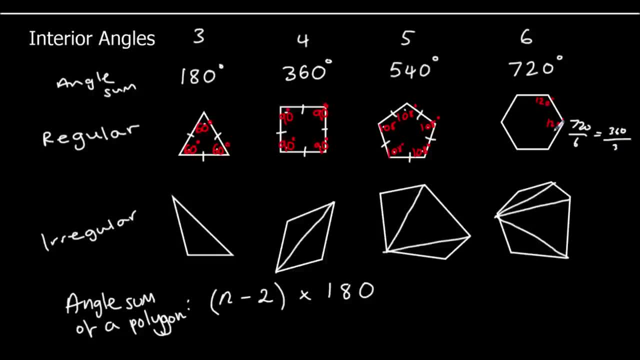 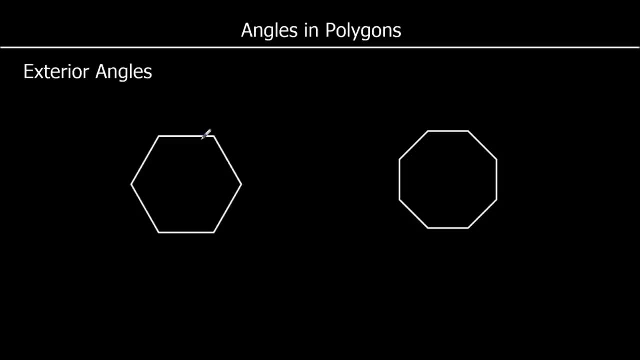 So we could say every angle in a regular hexagon is 120 degrees. Let's look at exterior angles now. So the interior angles are the ones inside the shape that we just looked at. The exterior angle is on the side And the interior angle is on the straight line with the interior angle. 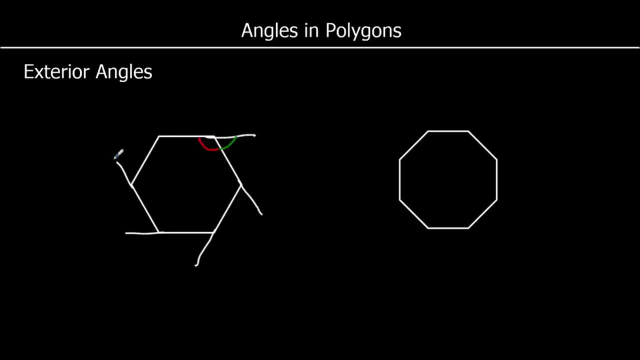 So the exterior angles and the interior angles are on a straight line, which means they add up to 180 degrees. So exterior angle plus interior angle equals 180 degrees. And we can also say that all of the exterior angles, So all of these green angles here, all of the exterior angles, add up to 360. 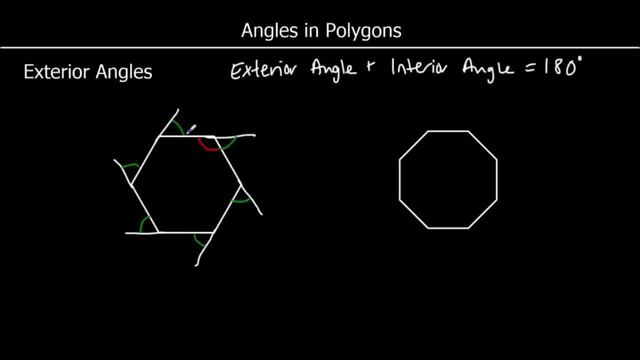 So if you walked all the way around the shape, you would have turned by all of these green angles And you would have gone around the whole way. You would have gone 360 degrees. So we also say Exterior angles, add to 360 degrees. 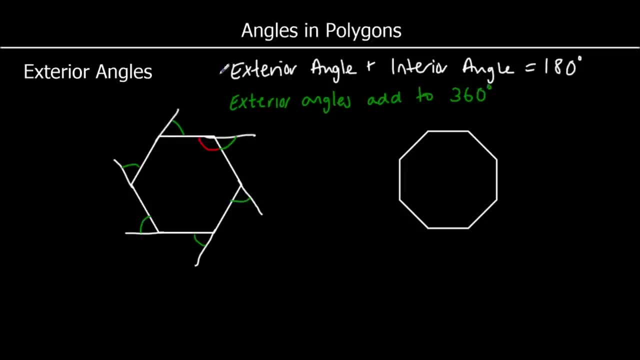 So here we've got a hexagon, a regular hexagon, So a six sided shape. We can find the size of each exterior angle by taking 360.. That's what they all add up to And dividing By six, because we've got six sides. 360 over six is 60.. 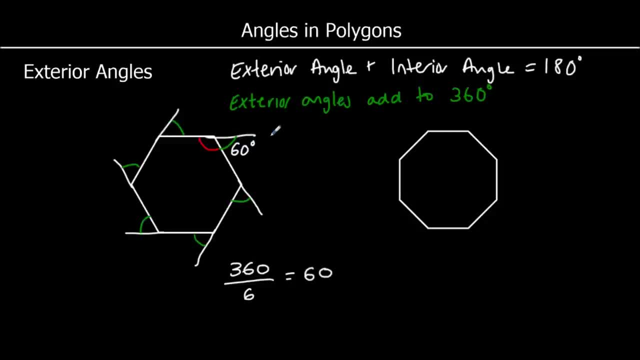 So we can say every exterior angle in a regular hexagon is 60 degrees And we can use this to find the interior angle as well, because we know they're on a straight line. So we can do 180.. Take away 60.. 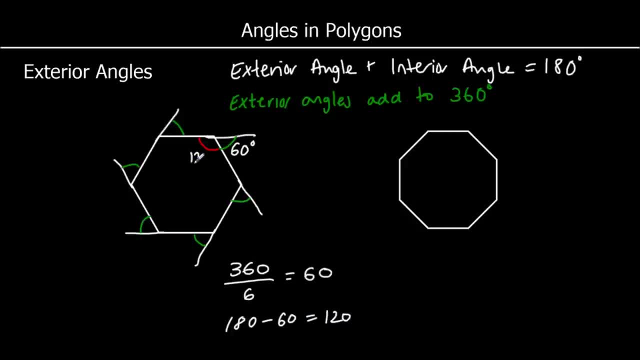 Which is 120.. So 120 and 60 add up to make 180.. For our eight sided shape We can say: the exterior angles always add up to 360 degrees. So 360 over eight is the same as 180 over four, which is the same as 90 over two. 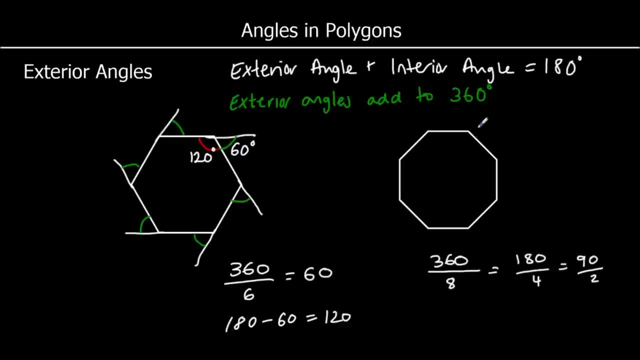 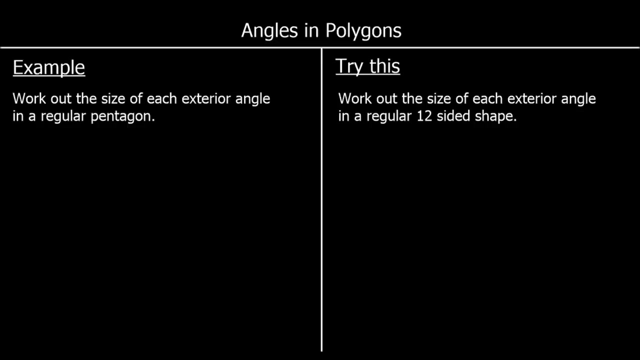 Which is 45. So the exterior angle is 45 degrees. So if we wanted the interior, 180 minus 45 is 135 degrees. Okay, Let's look at some questions. So the example Work out the size of each exterior angle in a regular pentagon. 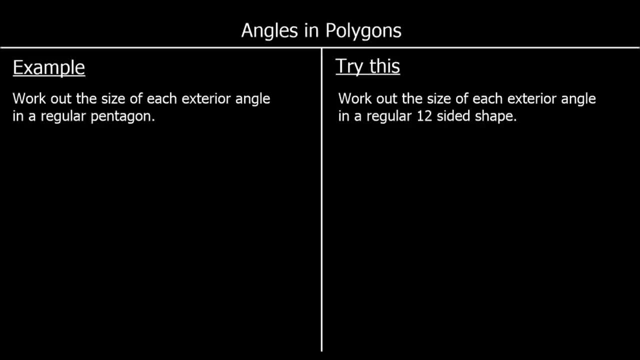 So the exterior angles, the ones on the outside, always add up to 360 degrees. A pentagon's got five sides, So it's 360 divided by five. How many fives go into 360? 360. So we can say that. 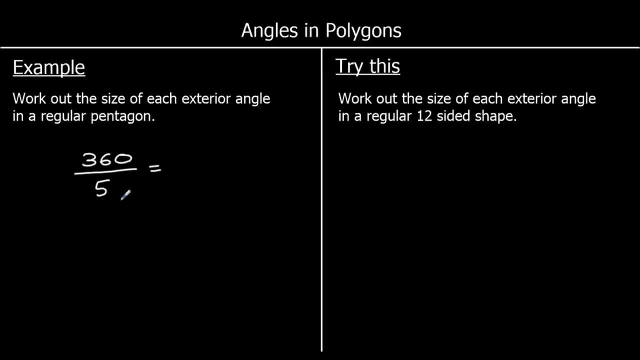 360 is 36 tens. do So double that, which is 72. So each exterior angle in a regular pentagon is 72 degrees. Okay, One for you to try. So give it a go. Work out the size of each exterior angle in a regular 12 sided shape. 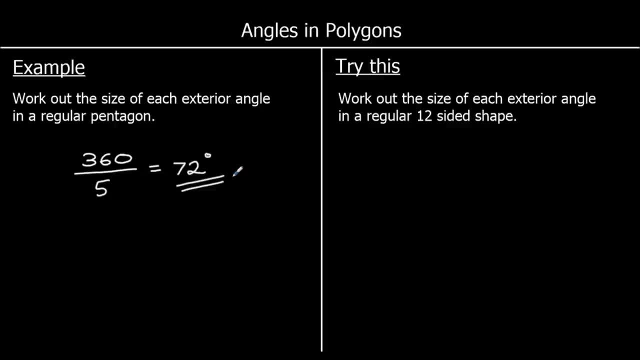 So a 12 sided shape is called a dodecagon And we We are. we are going to work this out by saying: the exterior angles always add up to 360 degrees and there are 12 of them, so 360 over 12. 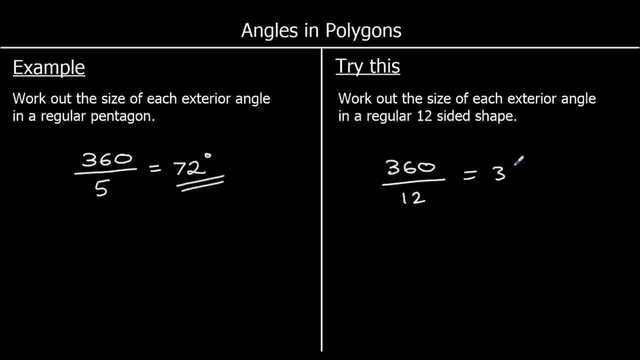 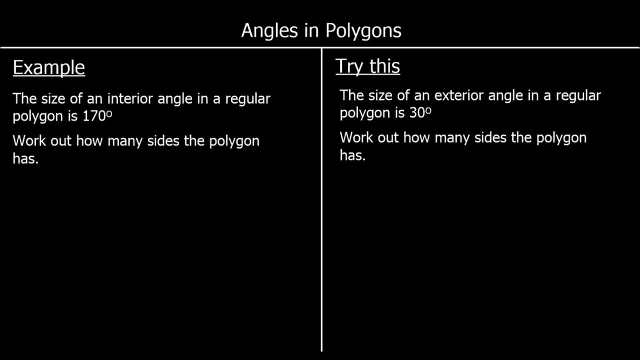 36 over 12 is 3, so 360 over 12 must be 30, so each exterior angle is 30 degrees. another example: the size of an interior angle in a regular polygon. so the inside angle is 170 degrees. how many sides does the polygon have? 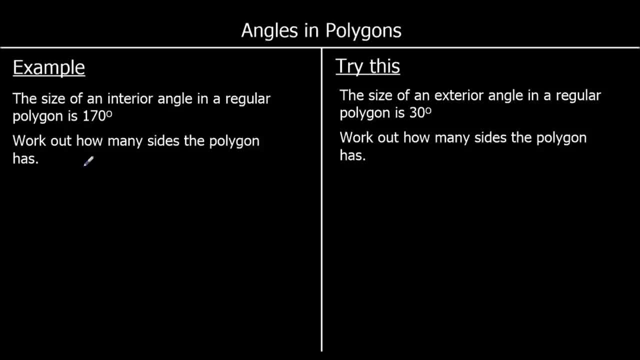 so the interior angle is 170, so the exterior angle is 170 degrees, is going to be 180. take away 170, which is 10 degrees, so we've got an exterior angle of 10 degrees and we know exterior angles always add up to 360. 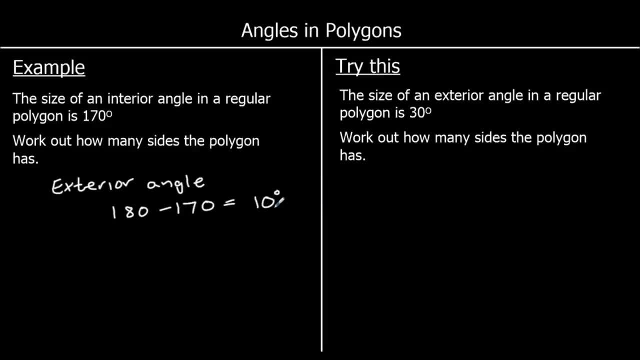 so how many 10s make 360?? so 360 over 10 is 36. so it's a 36. so it's a 36 and it has a 37 and it has a 37. so it has a 37 and it has a 37. 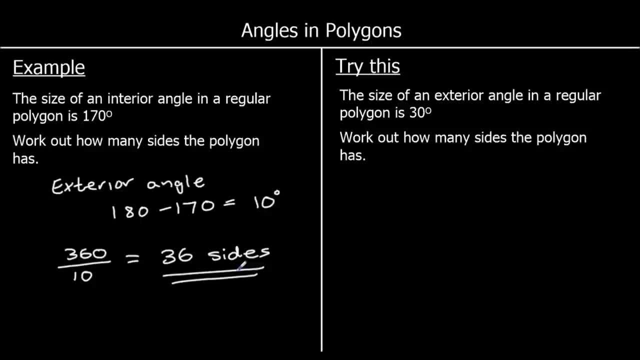 so if I add the two sides of the polygon it gets a 8, which makes it 17, which means the exterior angles always add up to 32 degrees. so the exterior angles make a 60, so it's a 36, so it's a 32. 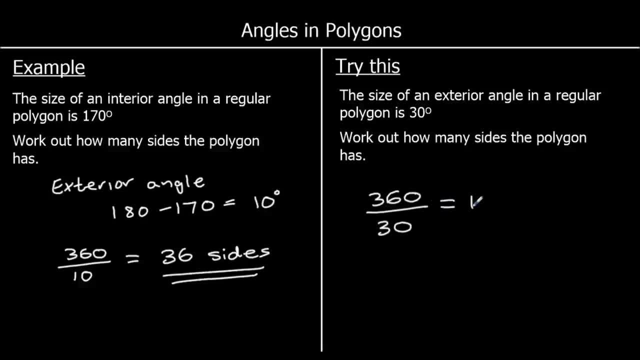 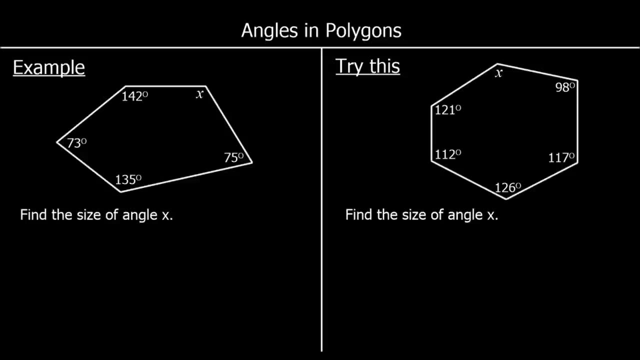 that is 12, so it's got 12 sides. okay, here's a different question. this time we've got irregular polygons, so all the lengths and all the angles aren't equal, but we're finding a missing angle. so let's look at how many sides we've got. we've got one, two. 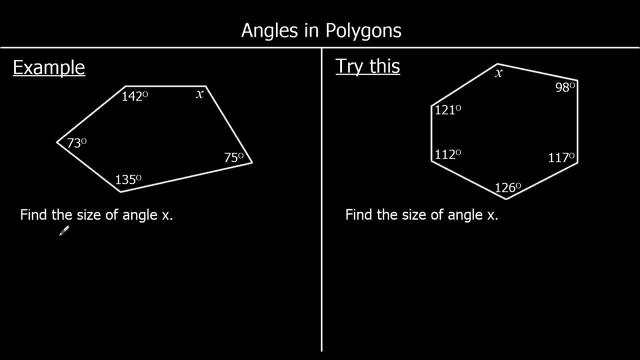 three, four, five sides. so we've got a five-sided shape, which is the pentagon. what do the angles in a pentagon add up to? so the angles in a pentagon add up to three times 180- remember it was n minus two times 180 for the angle sum. so three 180s is 540 degrees. so we need 540 degrees, all of these. 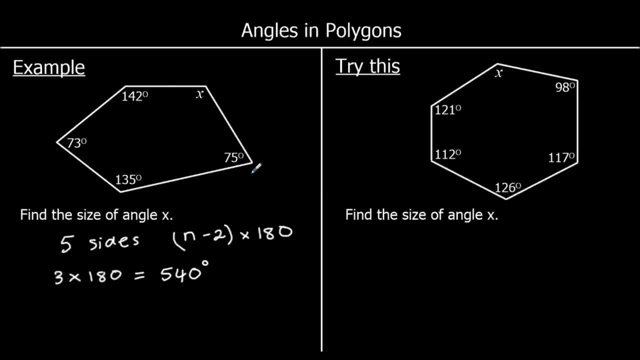 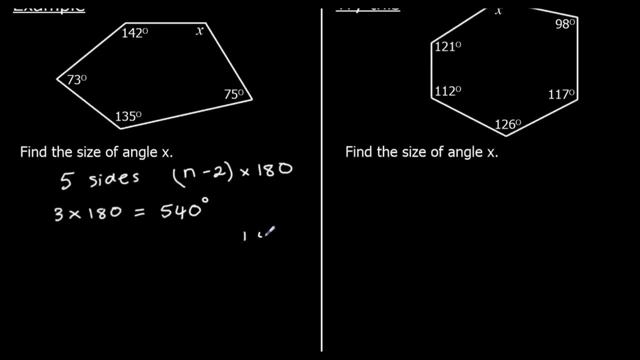 angles must add up to 540, so we're going to find a missing angle. so let's add up what we've got. we've got 142, 135, 75 and 73.. so let's add them up. five plus five plus two plus three makes fifteen. 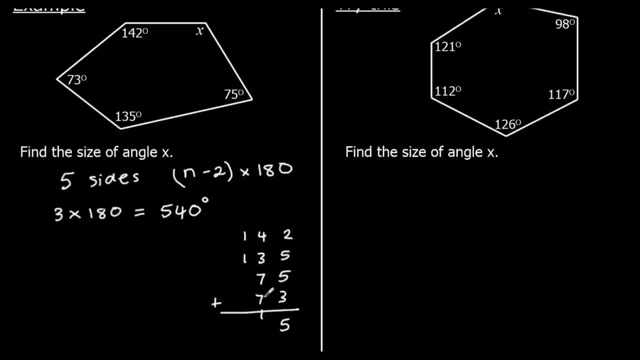 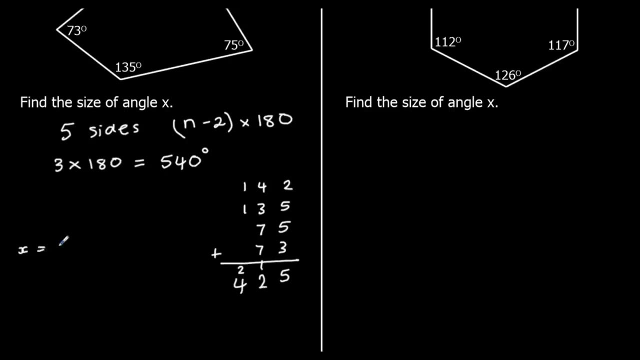 four plus three is seven. so seven plus seven plus seven is twenty. one plus one is twenty two, and one plus one plus two is four, so we've got 425 degrees so far. so x is 540. I take away 425, so that's one hundred and fifteen degrees. 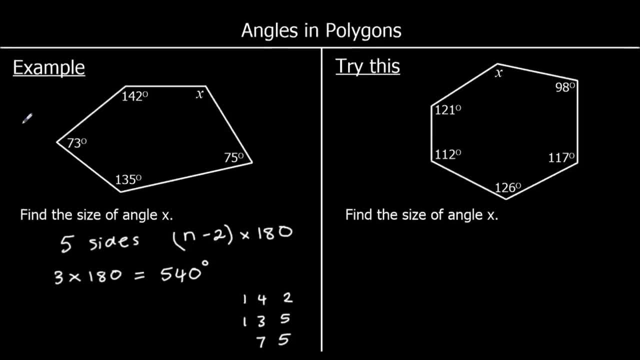 I am one for you to try, so give that a go. This time we've got a six side shape, so we can find 60 remain. the angles are supposed to add up to by doing 6 minus 2 times 180, which is 4, 180s, which. 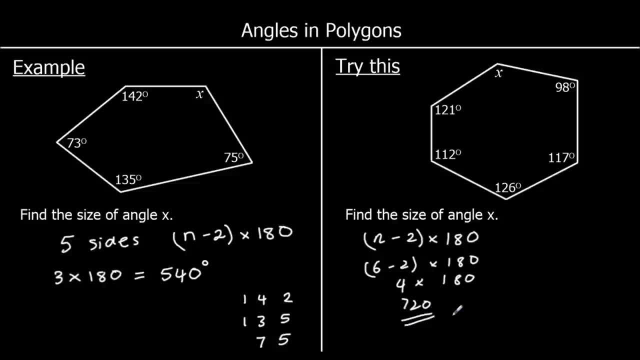 is 720.. So the angles have to add up to 720 degrees in a six-sided shape, in a hexagon, And let's see what we've got so far. So 126,, 121,, 117,, 112, and 98.. 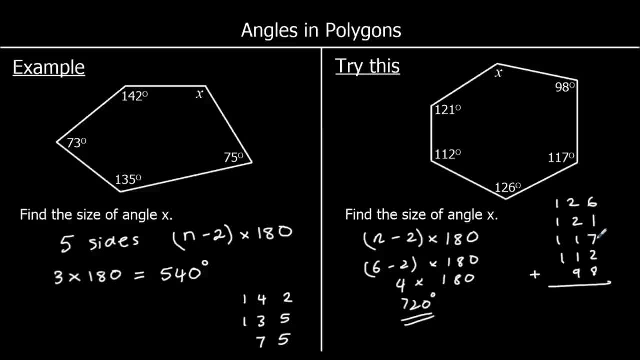 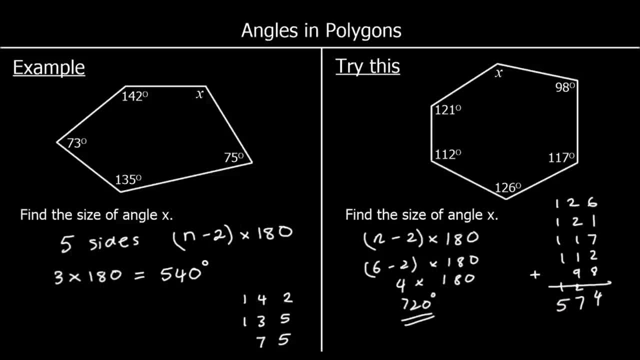 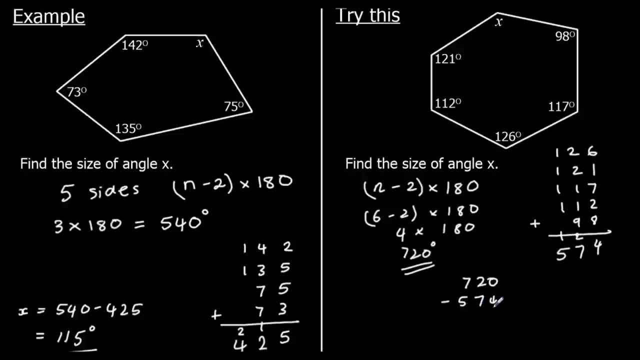 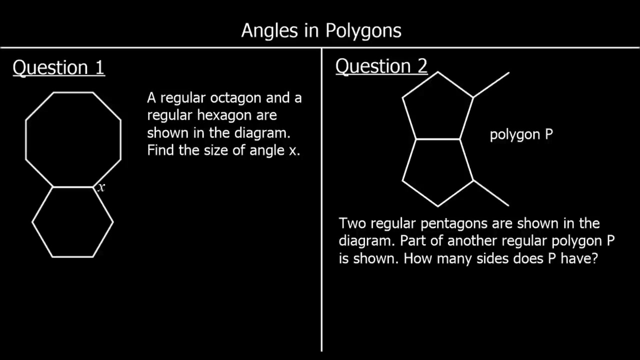 So we've got 574 degrees so far. 720 minus 574 is 146.. So x is 146 degrees. Okay, these are the last two questions. You can try and pause the video and answer them yourselves, or just keep watching for me to go through the answers. 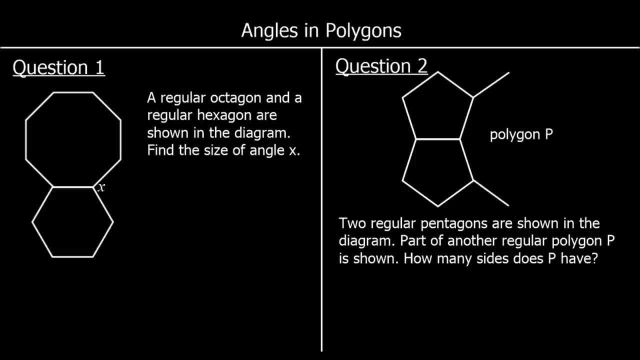 Question one: we've got a regular octagon, a regular octagon and a regular hexagon on the diagonal And we're looking for this missing angle x here. So we could either find the interior angle of the octagon, the interior angle of the hexagon. 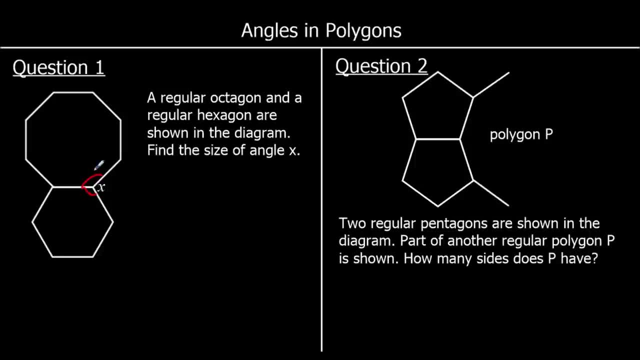 and then say the angles around the point, add up to 360 to find the missing angle. Or there's an easier way: If we split this x in half- well, not in half. if we split the x here, we can say we've got the exterior angle of an octagon plus the exterior angle of a hexagon. 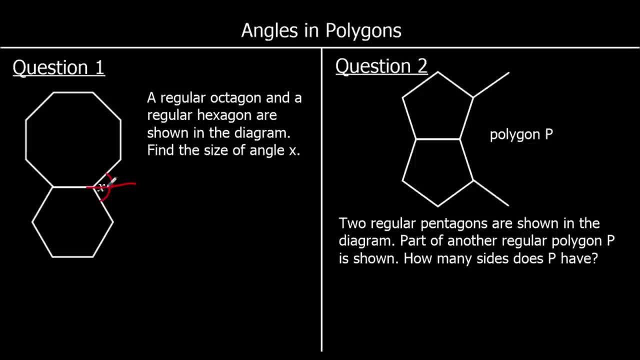 So we can find the exterior angle of an octagon by doing 360 over 8,, which is 45 degrees, And the exterior angle of a hexagon is 360 over 6,, which is 60 degrees. So angle x is 45 plus 60,, which is 105 degrees. 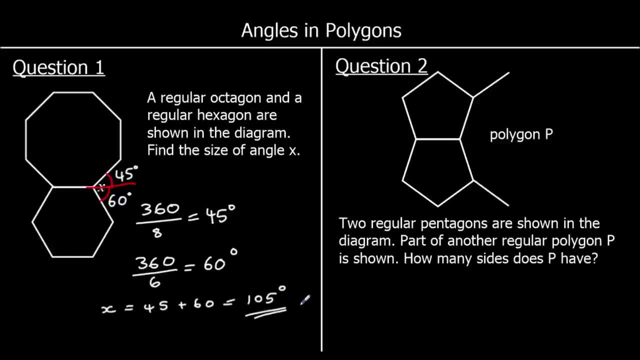 Question two: we've got two regular pentagons. in the diagram, Part of another regular polygon, P, is shown. How many sides does P have? So we are going to find, If we get the angles, the interior angles of the pentagons. 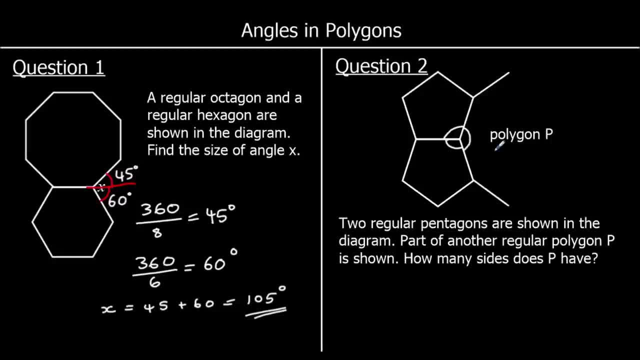 we can find the interior angle of the polygon P because angles around the point add up to 360 degrees. So let's do that to start. So each interior angle in a pentagon. So if I say the Exterior angle is 360 over 5, which is 72 degrees, 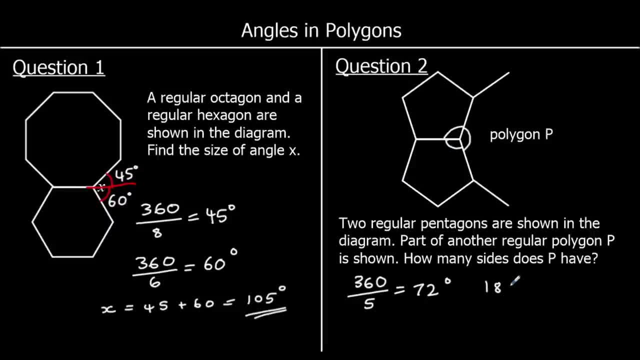 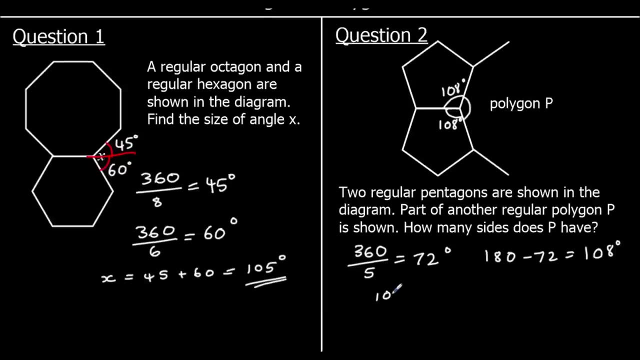 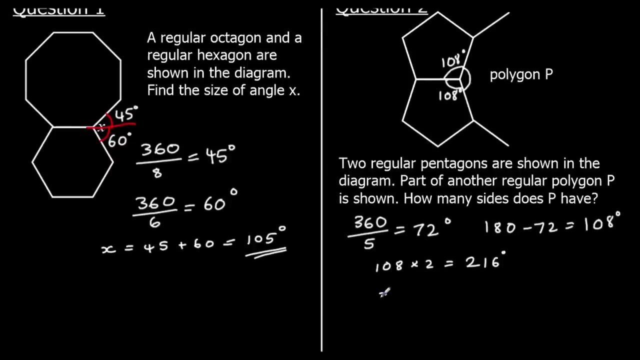 The interior angle is 180 minus 72,, which is 108 degrees. So we've got 108 and 108.. 108 plus 108 is 216 degrees, Which means well, we can find polygon P's interior angle by doing 360. take away 216, which will be 144 degrees. 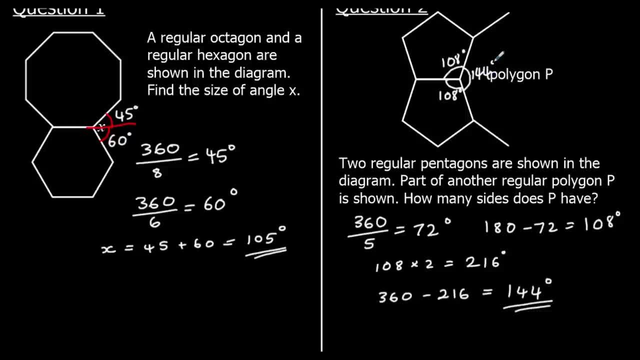 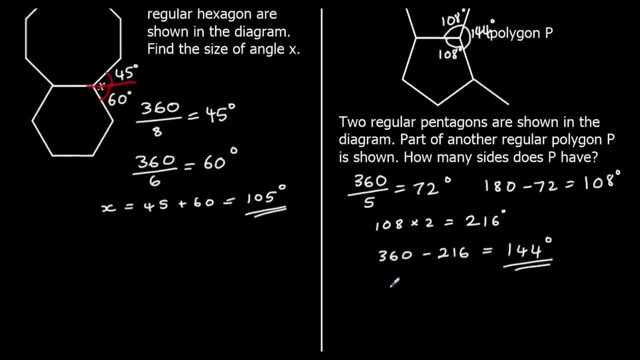